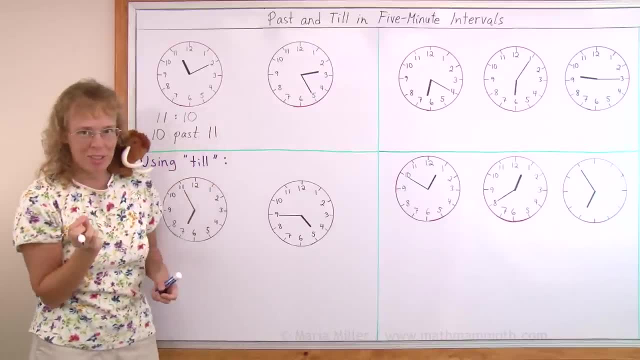 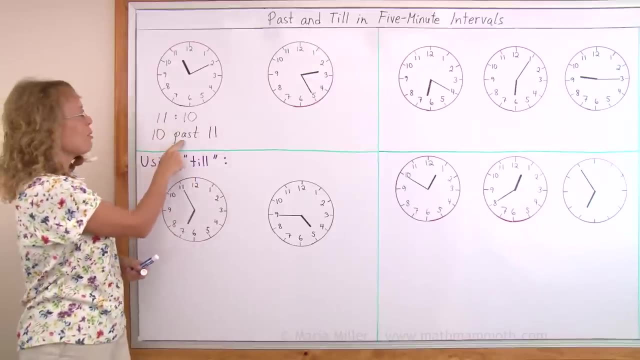 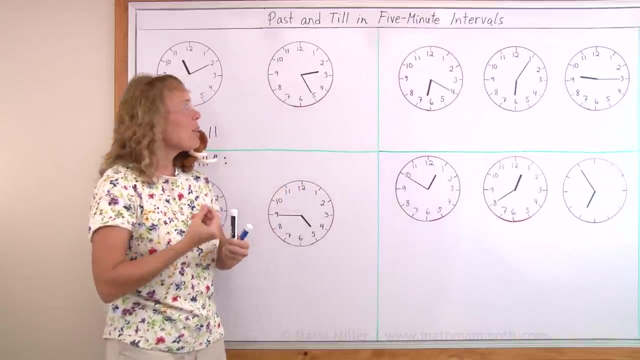 And that means 10 minutes past 11 hours. Okay, So it's pretty simple. It kind of looks like I switched the numbers 11 there and 10 there and put the word past in between. Let's try another one Over here. Let's just first write it the way we are used to You look at the. 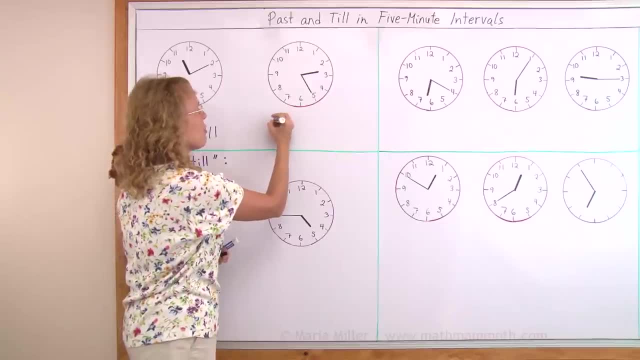 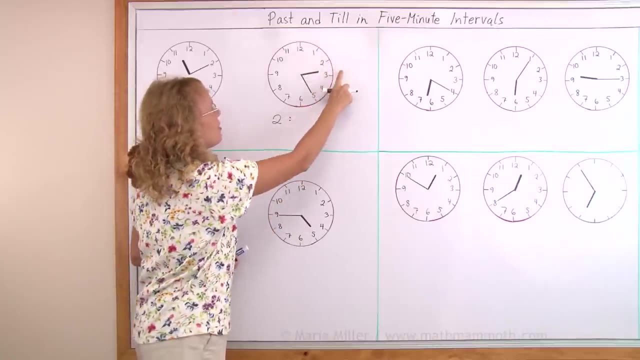 hour hand. so it is past two o'clock, two something two hours. And then the minutes. look at the minute hand over there count by fives. Five, ten, fifteen, sixteen, eighteen, twenty, twenty-two, twenty-three, twenty-three, twenty-four, twenty-five, twenty-six, twenty-seven. 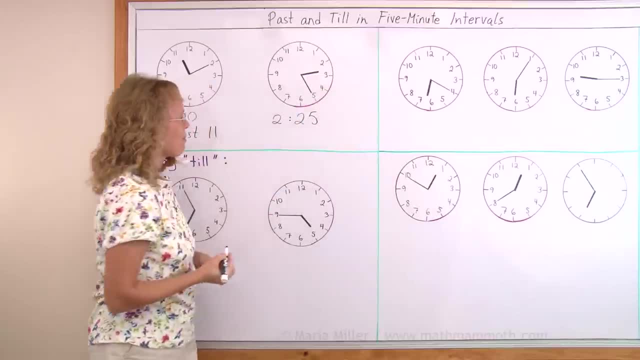 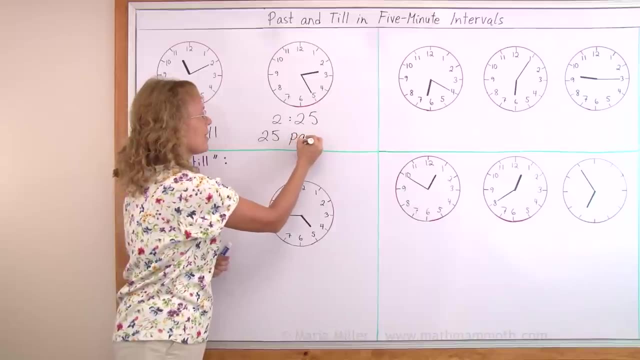 twenty-seven, twenty-eight, twenty-nine, twenty-nine, twenty-eight, twenty-nine, twenty-nine, twenty-nine, twenty-nine, fifteen, twenty, twenty-five, Two, twenty-five. And now the other way of saying it: we will say the minutes first, How many minutes it is past the whole hour. Twenty-five past two. 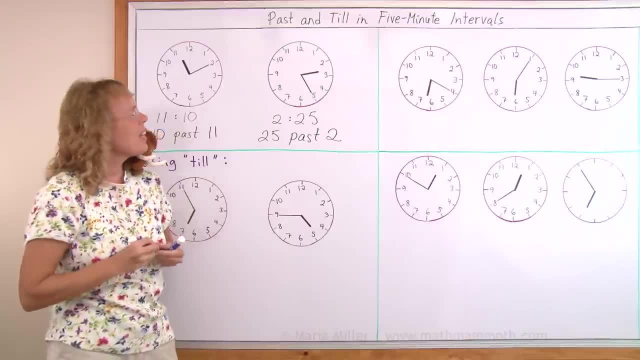 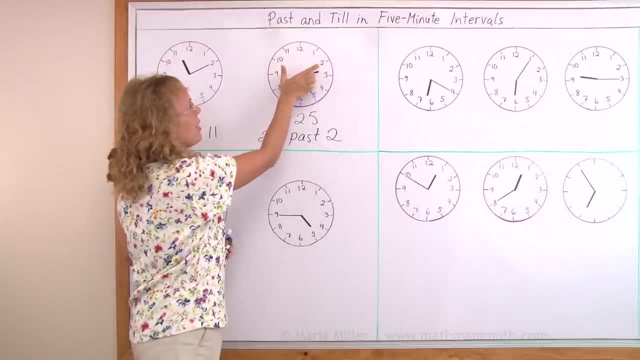 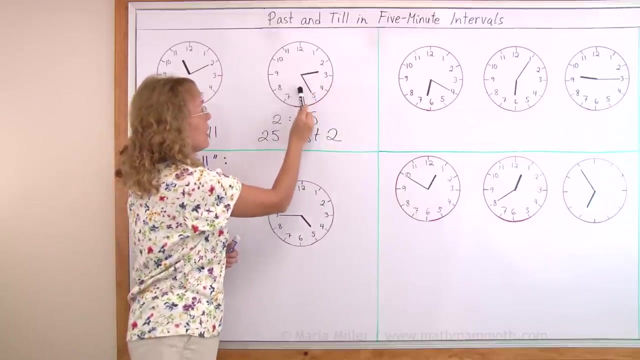 Or you can say twenty-five minutes past two, And we will use this past whenever the minute hand is here: Five past something, ten past fifteen past, or twenty past, or twenty-five something Up to when. it is right here, pointing straight down which is the half past, The. 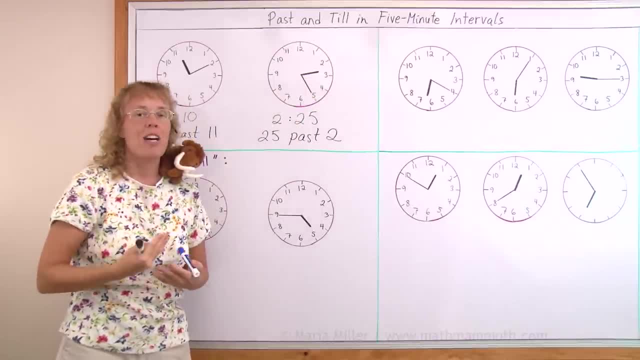 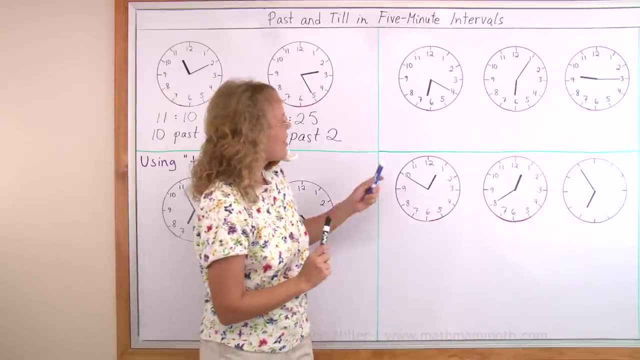 half past actually is thirty minutes past the whole hour, but we will say it as half past the whole hour. Now we are going to just do a few more exercises, But before I tell you those, why don't you pause the video and try them on your own? 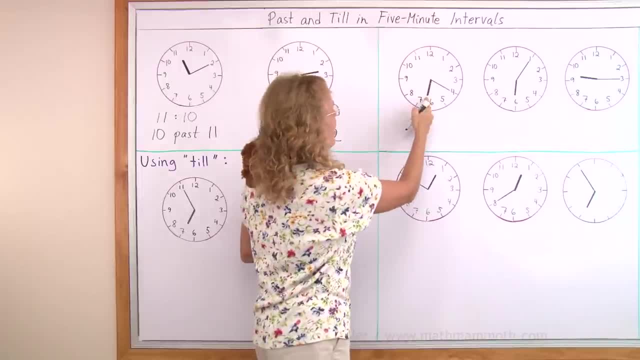 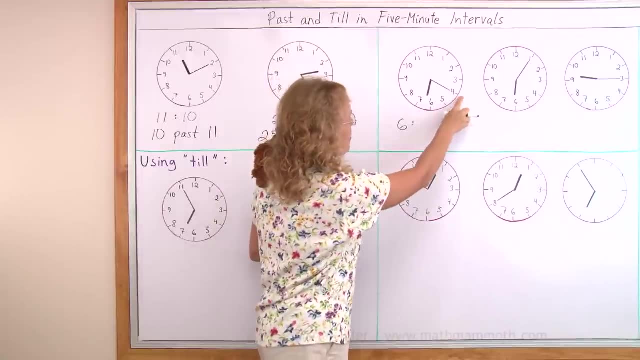 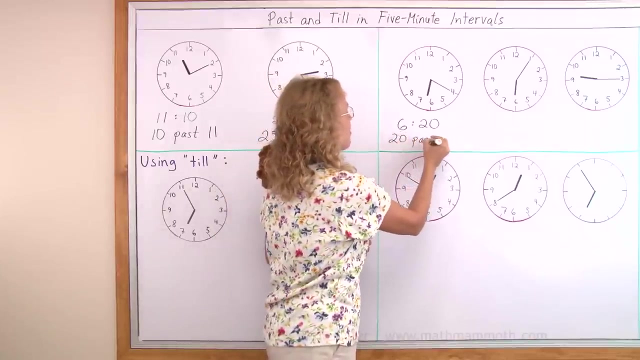 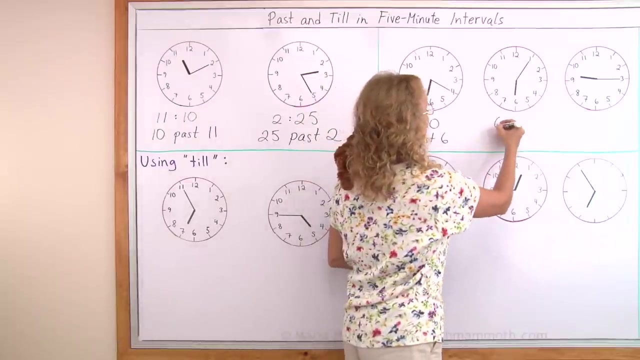 Okay, now this one. look at the hour hand over here Between six and seven. so it is six hours, right? And the minutes can you tell? Twenty, Six, twenty And the other way of saying it, twenty past six Over here. hour hand at six Again, Minute hand: just five minutes, okay, Six. 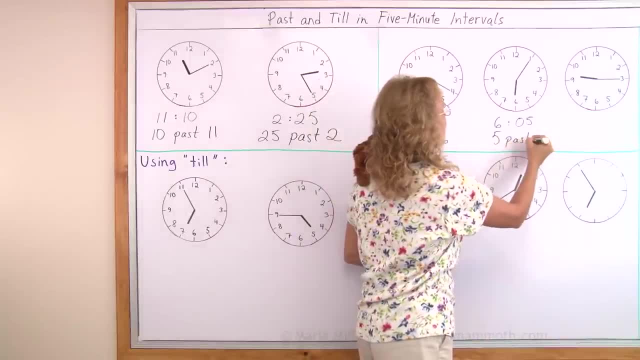 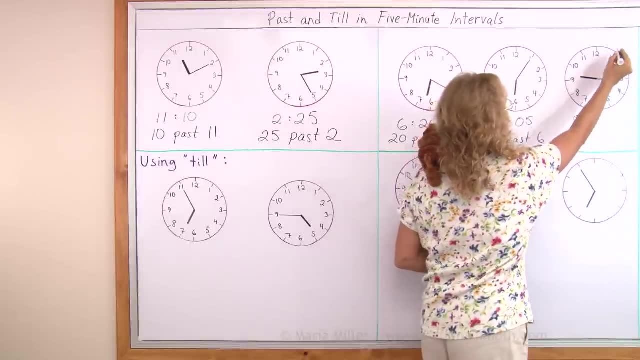 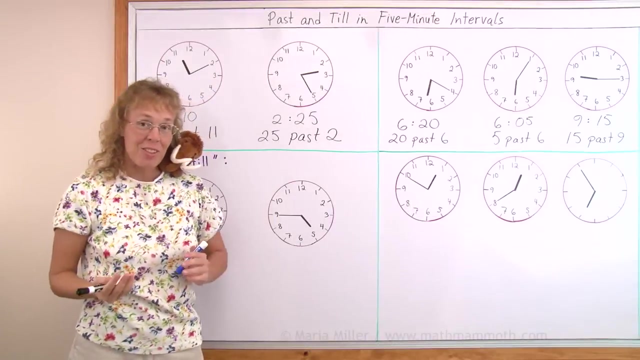 o' five or five past six. The last one, for now Hours are nine and the minutes fifteen, So it is fifteen past nine. And now the other one. I told you about using the till, which is a little bit more tricky. 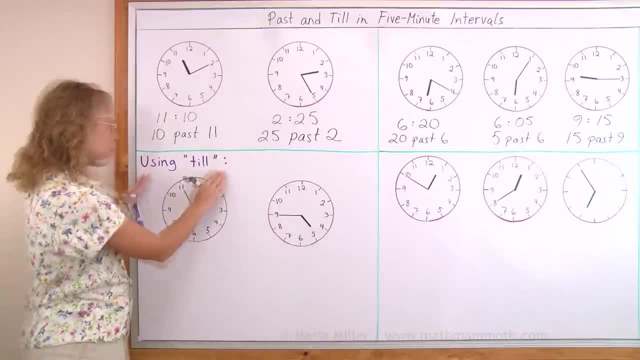 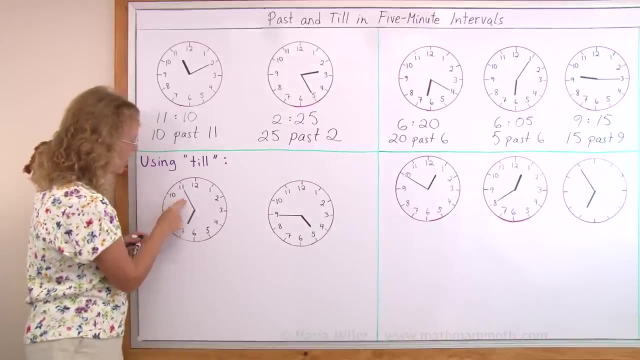 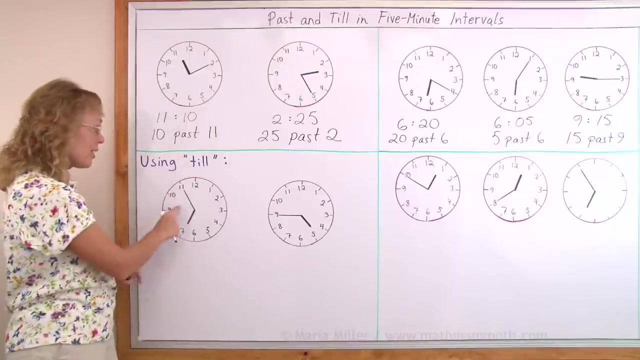 But let's look at it. We use the word till to say how many minutes till the next whole hour. For example, here the minute hand is just five minutes till the next whole hour, which is seven hours. So this time is five till seven, Five minutes till seven hours. 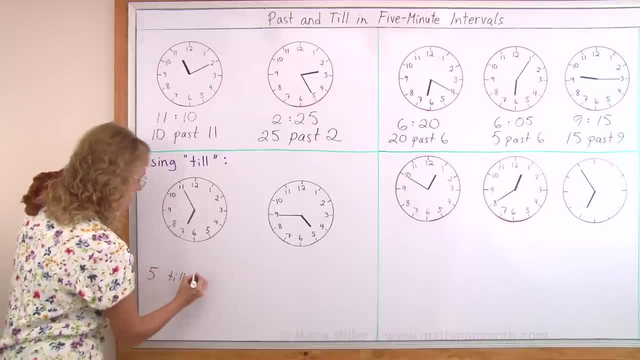 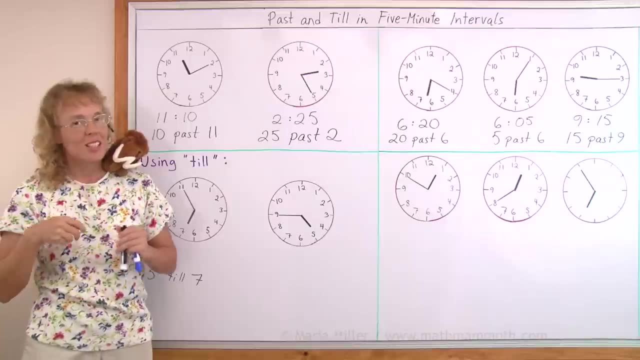 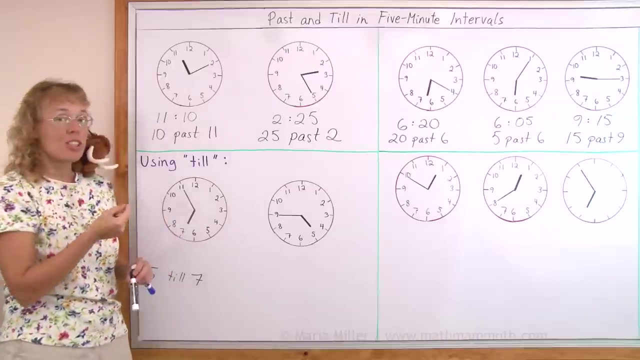 So let me write it here Now. the usual way of saying this that you already know is actually a bit more difficult, Because for that, if you remember, we were looking at the hour hand and we figured that it's not yet seven o'clock. 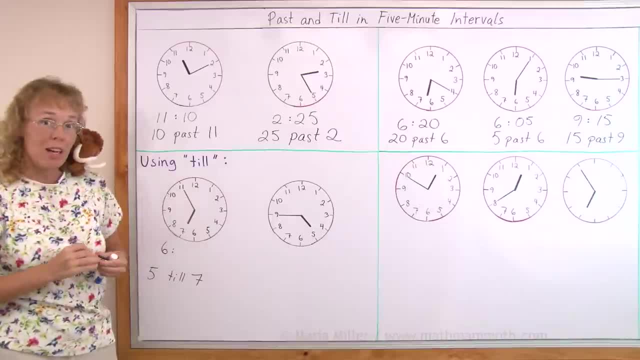 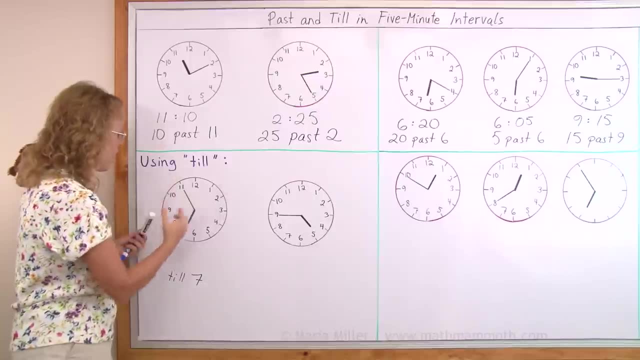 So it is still six hours something. And then we counted by fives, remembering here is thirty minutes: thirty-five, forty, forty-five, fifty, fifty-five, This was six, fifty-five, And it is also five minutes till seven. 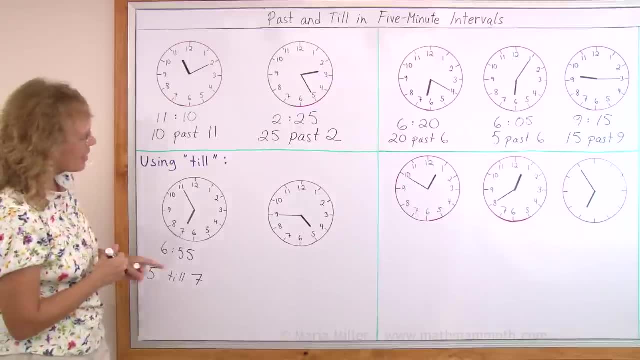 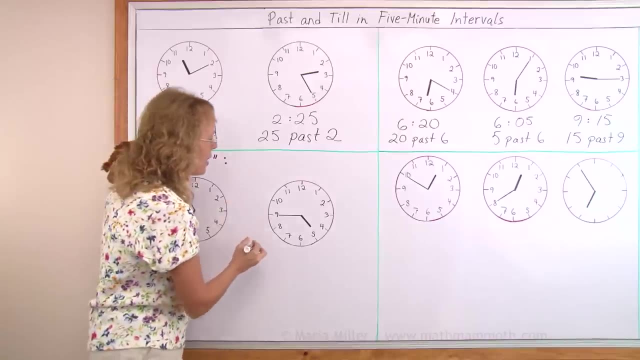 So these two look really different from each other. right, Let's look at here. We will figure out how many minutes till the next whole hour? How many minutes does the minute hand need to move to get all the way up here to the? 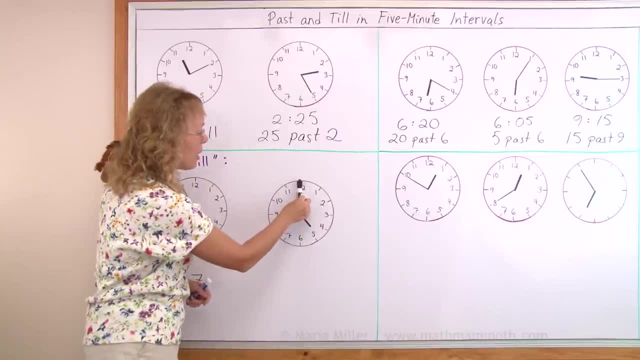 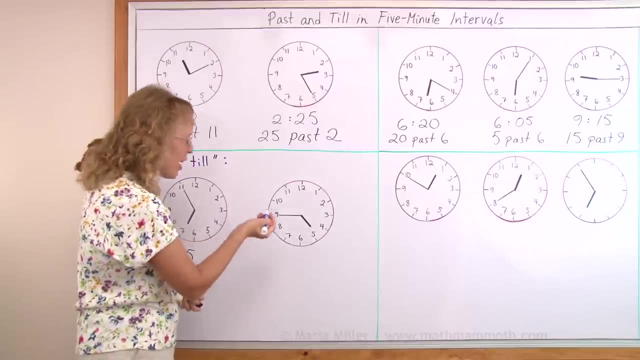 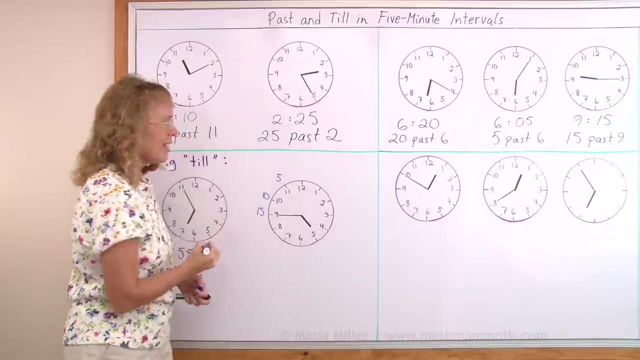 next whole hour, Which the next whole hour when it is up here. then you will have exactly five o'clock. But how many minutes till five o'clock? You can, for example, count by fives backwards from here, like this: Five, ten and fifteen. 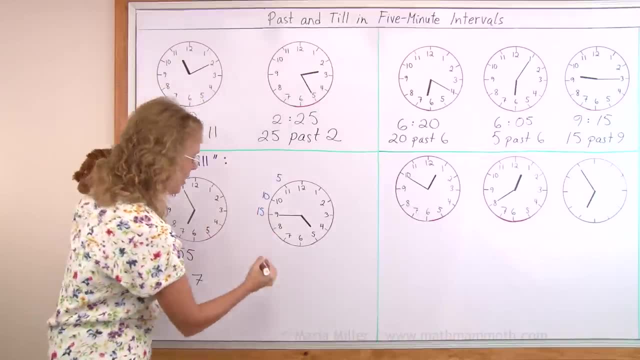 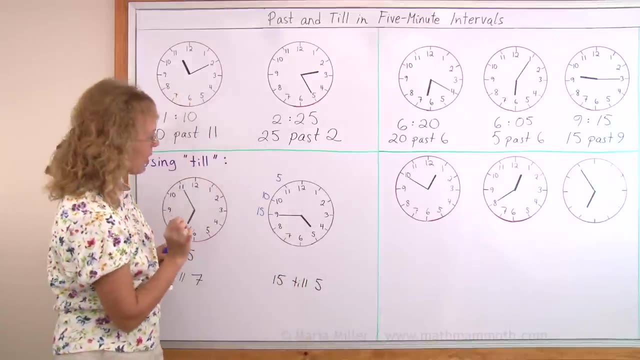 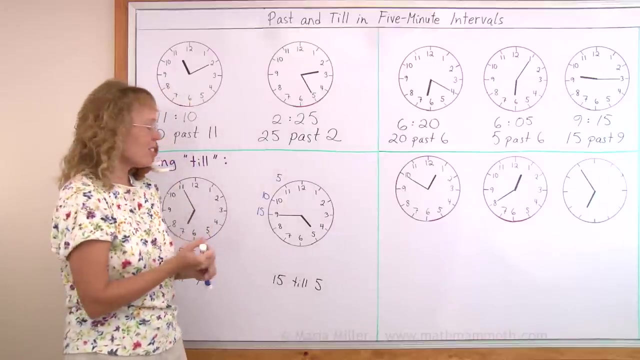 And figure out. it's fifteen minutes till five. Let me write it here And now. the other way of saying the same time was that we say hours and then minutes till five minutes. Okay, And for that it's not yet five o'clock, so it's still four hours, And 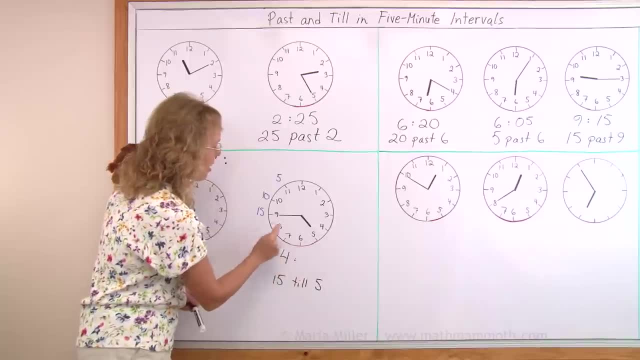 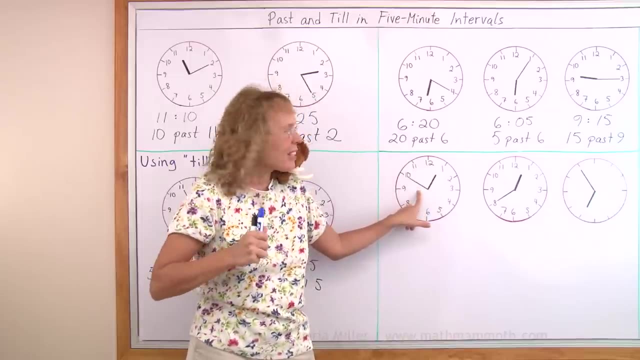 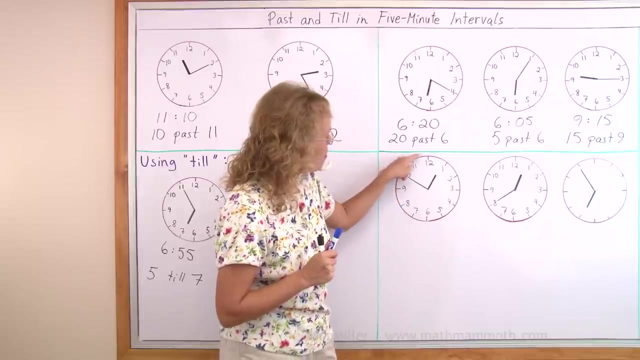 the minutes counting by fives: 30,, 35,, 40,, 45.. Here's the minute hand: How many minutes till the next whole hour And what is the next whole hour? Okay, the minute hand needs to move two steps, so to speak. So that makes 10 minutes because you count by fives. okay. 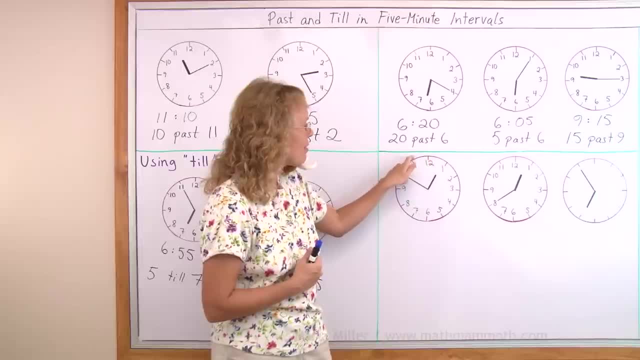 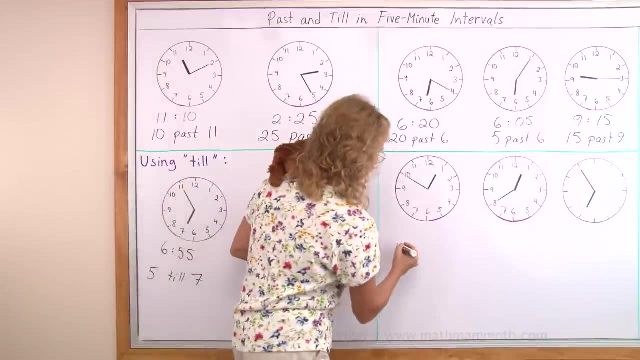 Five and 10.. Or you can count from here: Five and 10, either way, So 10 minutes till. but what is the next whole hour? The hour hand is almost coming to one, so it is one 10 till. 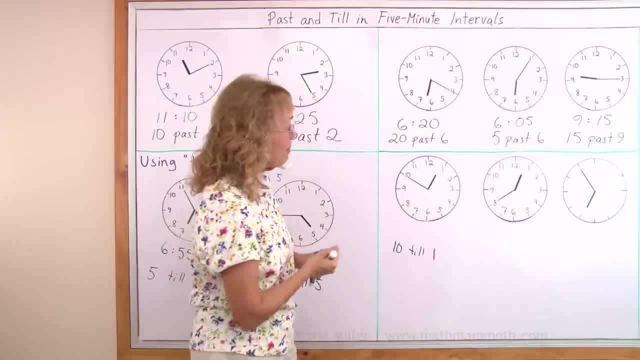 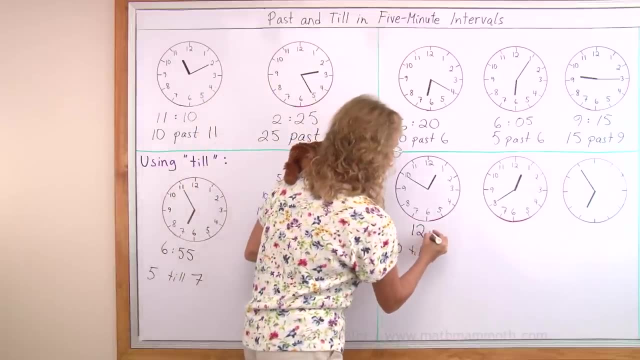 one And the other way of saying it. since it's not yet one o'clock, we will have to say it is 10.. 12 hours and so many minutes, Okay, 12.. And counting by fives, if here's 30 minutes, 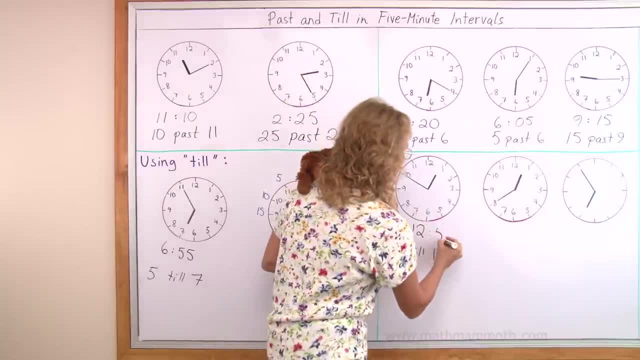 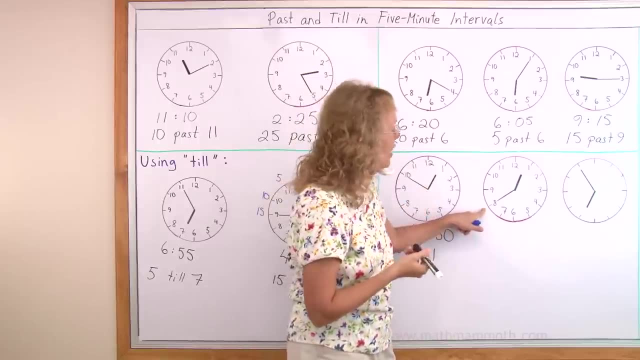 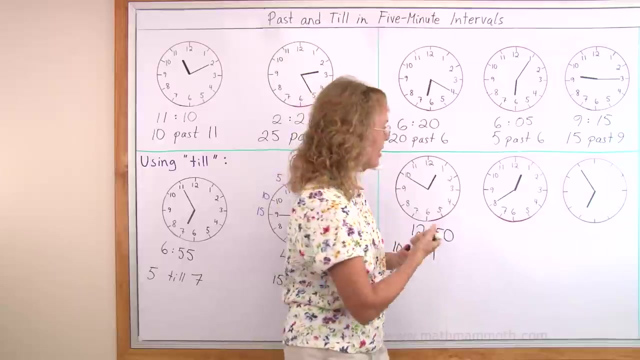 35,, 40,, 45, and 50.. 12,- 50. Over here. minute hand is here. How many minutes till the next whole hour? Okay, We count by fives, Five: 10,, 15,, 20.. 20 minutes till. till what hour? 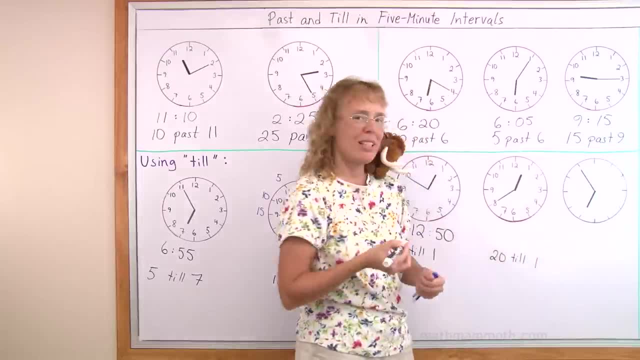 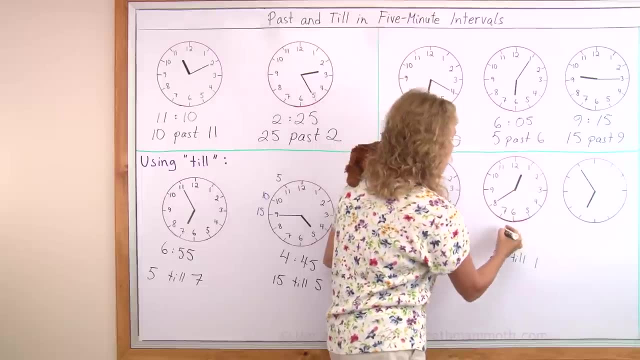 One. The hour hand is going to be at one, so 20 minutes till one, And then the other way again. it is not yet one o'clock, it is just 12 hours, and then 30,, 35,, 40,, 40. 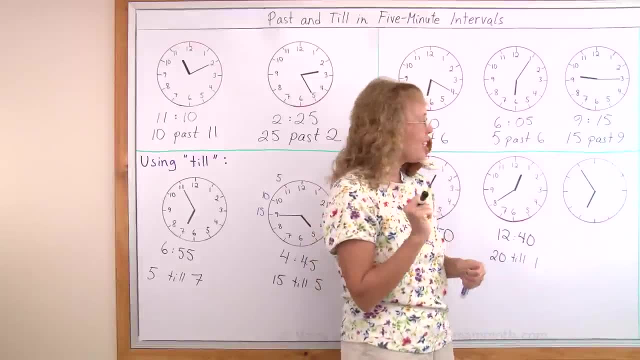 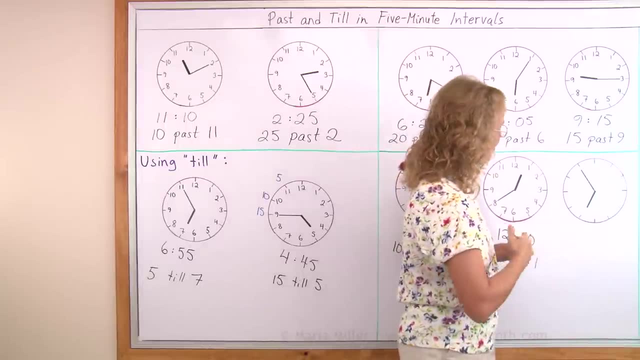 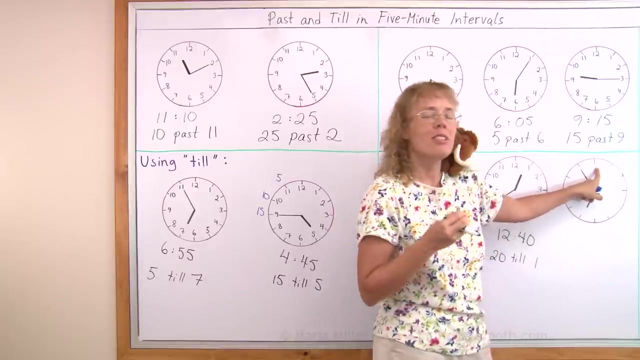 minutes. The last one is a little bit of a challenge because we don't have the numbers on the clock face. okay, Can you figure out what time it is? This is the hour hand. this is the minute hand. Notice, the minute hand has just one step to go till the next whole hour. So it is just 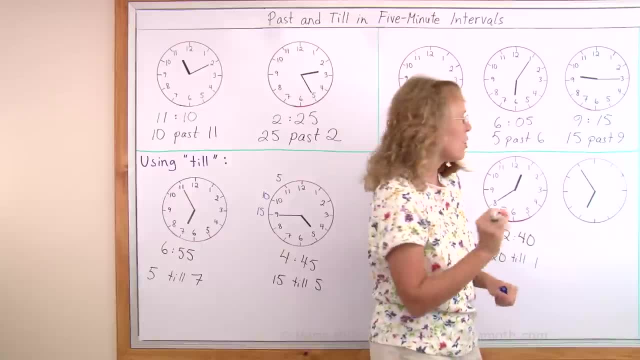 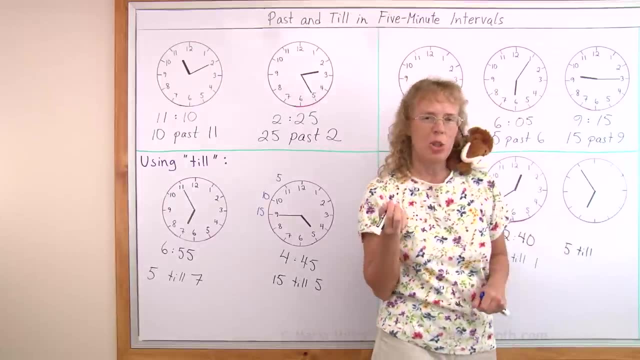 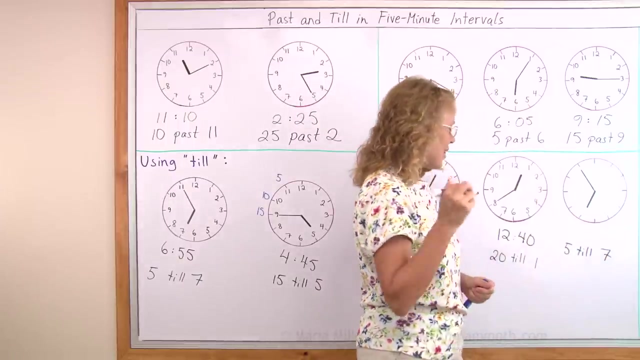 it's not one minute till something, it is five minutes till, because one step here means five minutes. It is five minutes till the next whole hour. What is the next whole hour? The hour hand is going to be at seven, And the other way of saying it, since it's not. 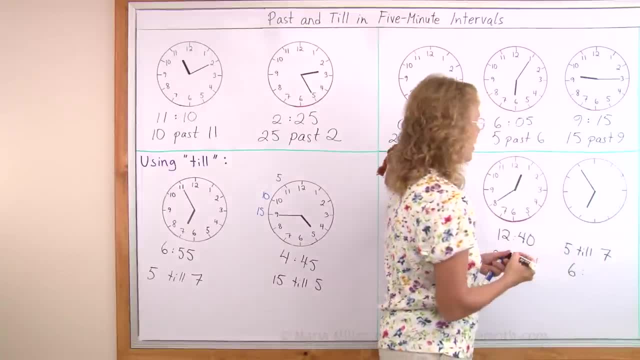 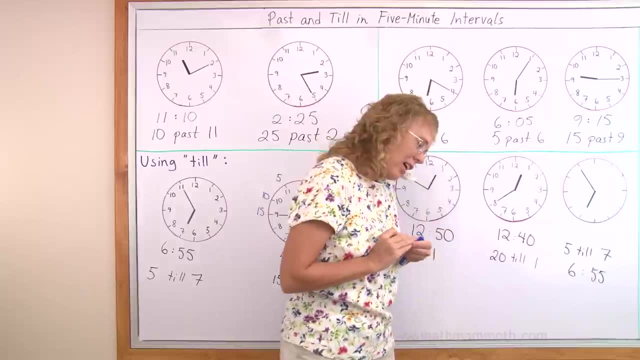 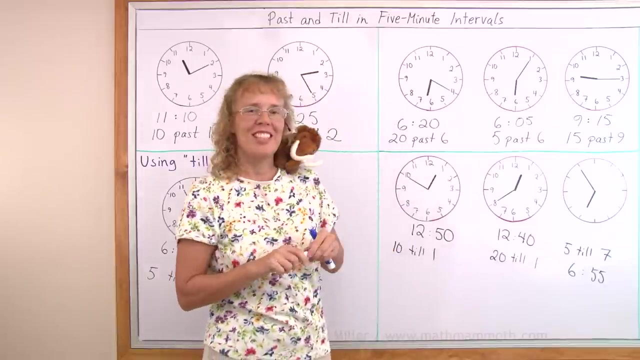 yet seven hours. it is till six hours, something Okay, And if you remember, over here will be 55 minutes. Mmhm, Matti has a challenge for you. just wait a second. What time is it if it is 55 minutes?